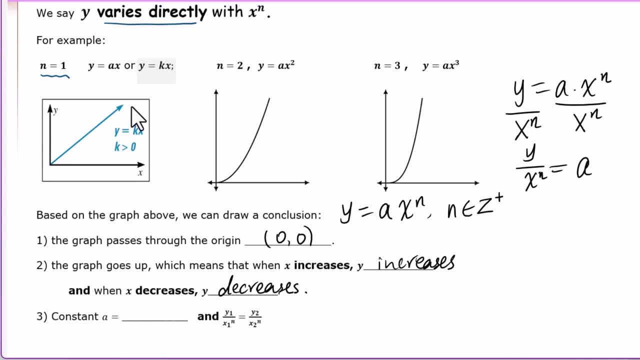 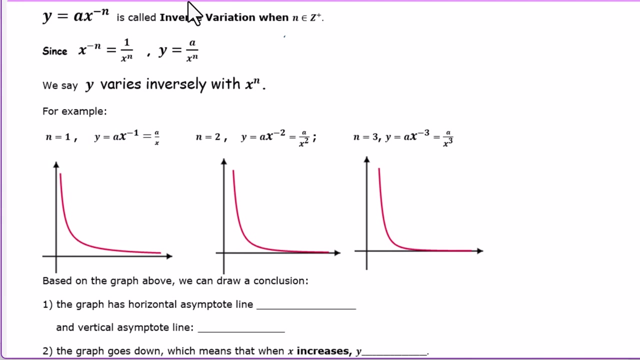 t over x to the nth power. Now also, y1 over x1 to the nth power equals y2 over x2 to the nth power, because the both equals a constant a For inverse variation. y equals a times x to the negative nth power. n is a positive integer Since x to 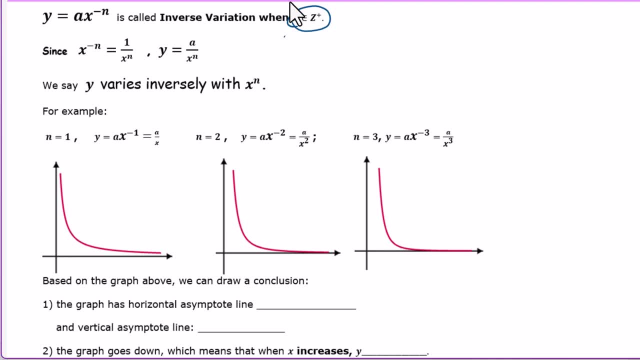 the negative nth power equals 1 over x to the nth power. we can write inverse variation into: y equals a over x to the nth power. We see y varies inversely with x to the nth power. Let's look at some graphs. When n equals 1, the graph is this: 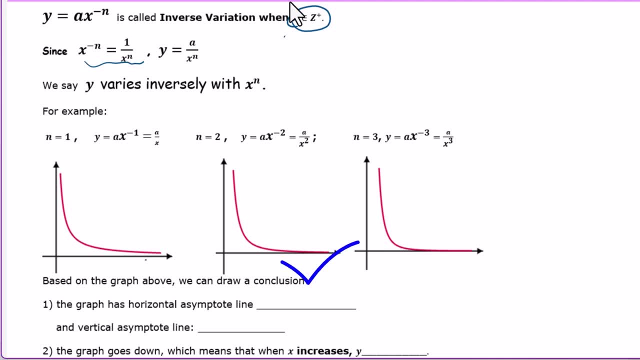 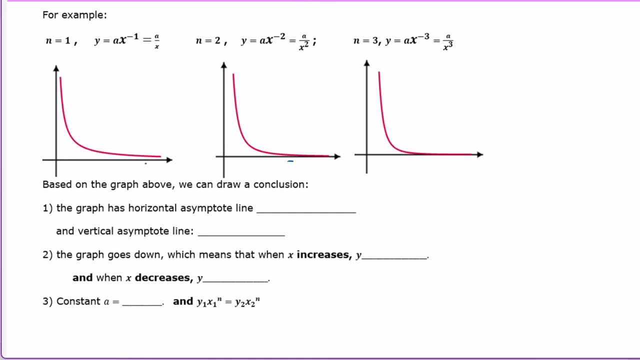 When n equals 2,, the graph is this: When n equals 3,, the graph looks like this: Based on the graphs above, we can draw a conclusion for: y equals a times x to the negative nth power. also equals a over x to the nth power. The graph has a: 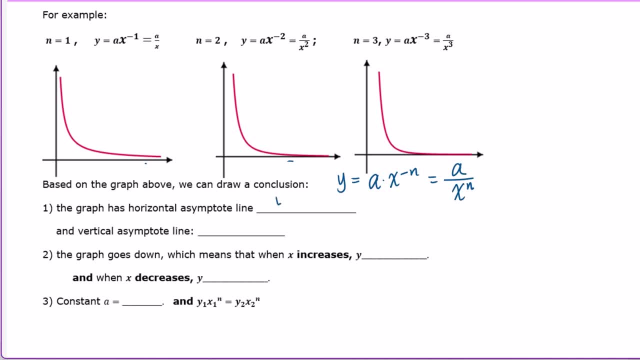 horizontal asymptote line y equals 0.. Also it has a vertical asymptote line x equals zero. The graph goes down, which means when x increases, y decreases the power, х goes down. fine, Just say the wrong 95, Heart 2, it goes down. still the first 0 in x increases, y decreases. 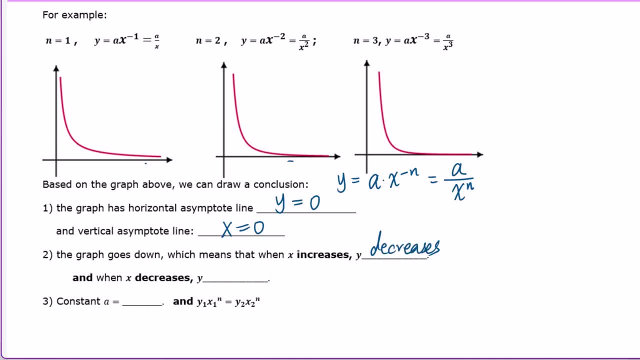 and a right part of: 5 times 2 equals 2, and the organizers comma and the number of both times x and 0. iRock between those two. And when x decreases, y increases, Constant number A equals. We know y equals A over x to the nth power times x to the nth power, both sides. 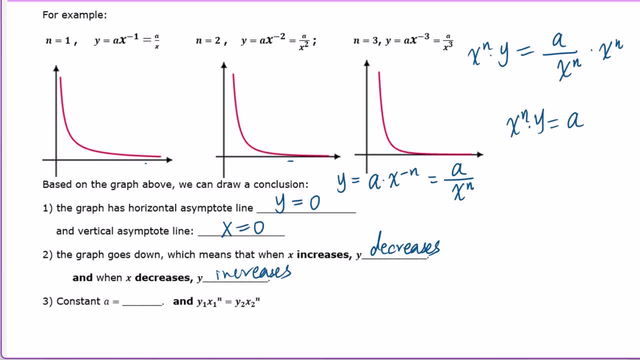 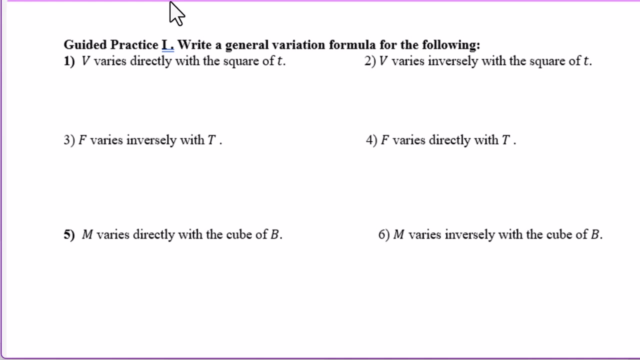 A equals x to the nth power times y. Also, we have y1: x1 to the nth power equals y2 times x2 to the nth power, because both equals constant A. Write the practice. 1.. Write a general variation formula for the following: 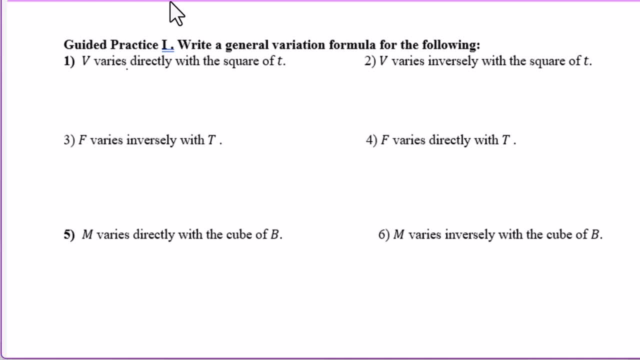 Question 1.. V varies directly with the square of t. Directly Directly Means positive exponent. So we have t to the second power. V equals A times t to the second power. A is a constant. Question 2.: 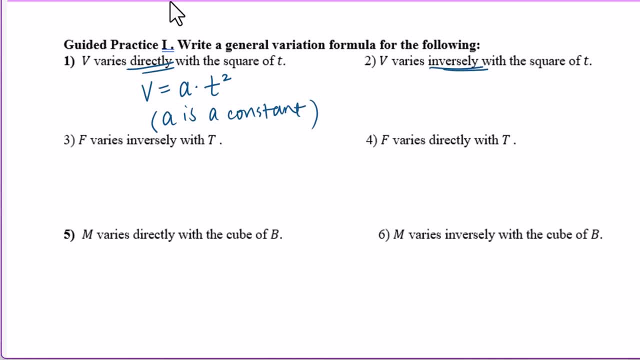 V varies inversely with the square of t. Inversely means negative exponent T to the negative second power. V equals A times t to the negative second power equals A over t. squared A is a constant. Question 3. F varies inversely with t. 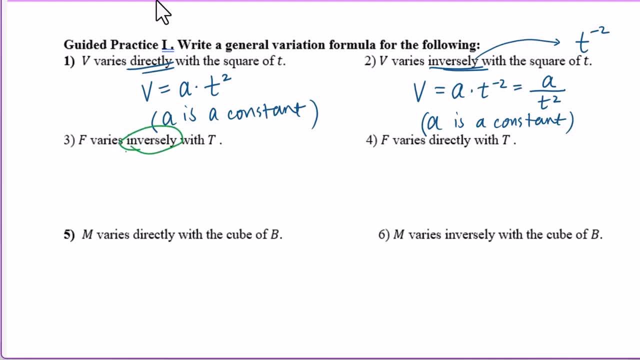 Inversely means negative exponent, T to the negative first power. So F equals A times t to the negative first power, Which means A over t. A is a constant Question. 4. F varies directly with t. Directly means positive exponent. 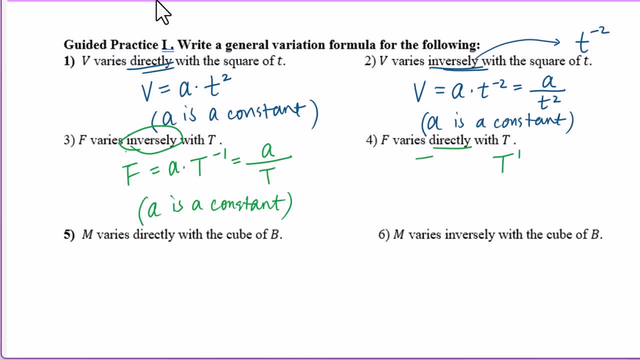 So t to the first power, F equals A times t. A is a constant Question. 5. M varies directly with the cube of b. Directly means positive exponent B to the third power. M equals A times b to the third power. 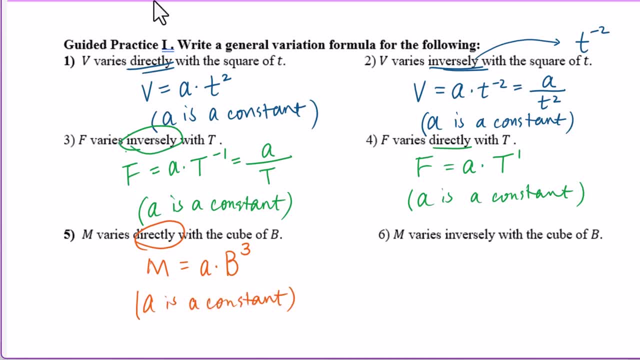 A is a constant. M varies inversely with the cube of b. Inversely means negative exponent B to the negative third power. M equals A times b to the negative third power. equals A over b to the third power. A is a constant. 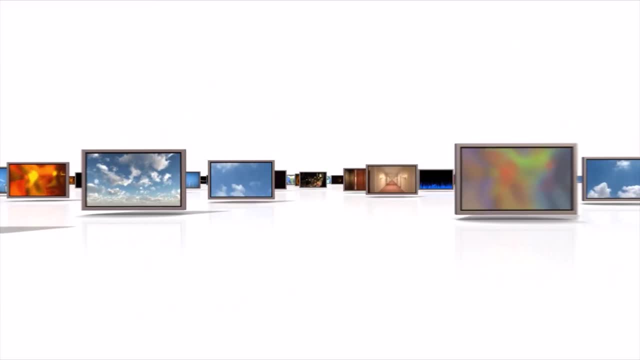